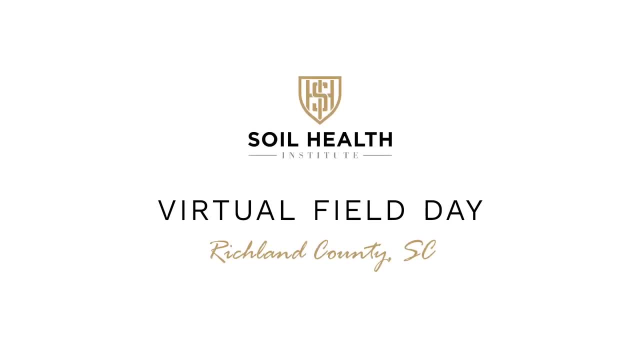 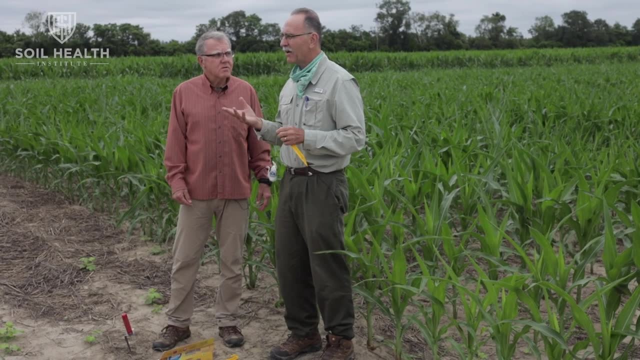 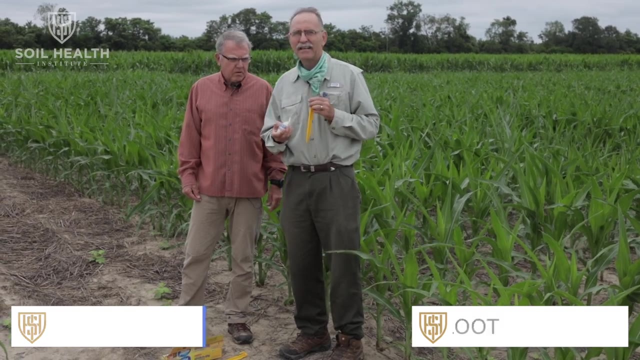 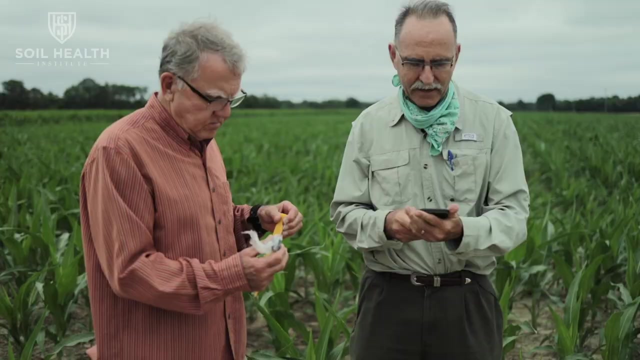 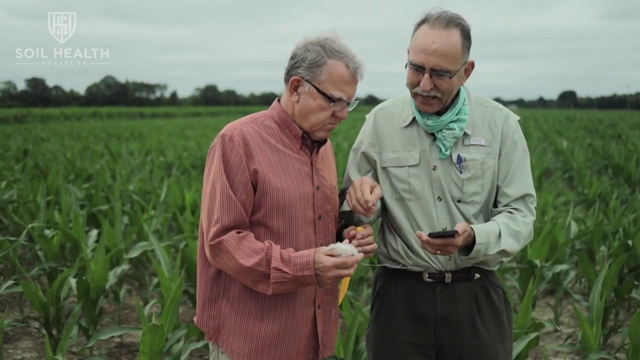 Okay, we're going to look at soil temperature. today, Of course, it's not exactly hot, But this is a pendant. Basically, it's a Bluetooth connected pendant And, if you hold this for me, David, I actually have an app on my phone And this pendant- now actually the app's. 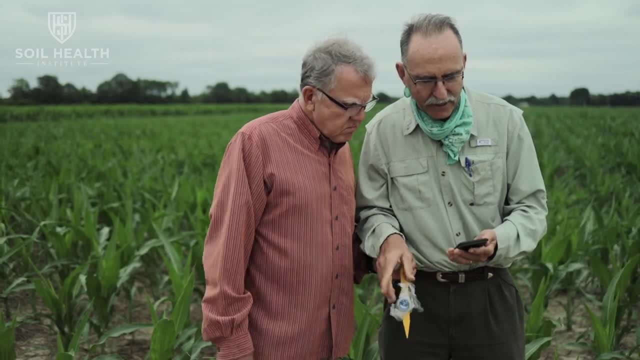 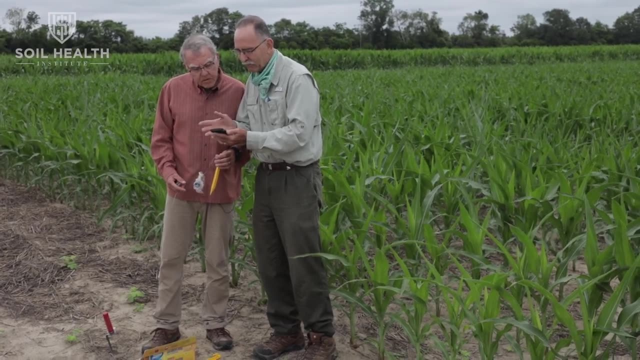 been programmed And I'm just going to click the middle here And there you go. That is NCO2, right? Yes, And so you can see we've got a temperature of 80.03.. And if we look at it, we'll also be able to see whether it's recording or not. 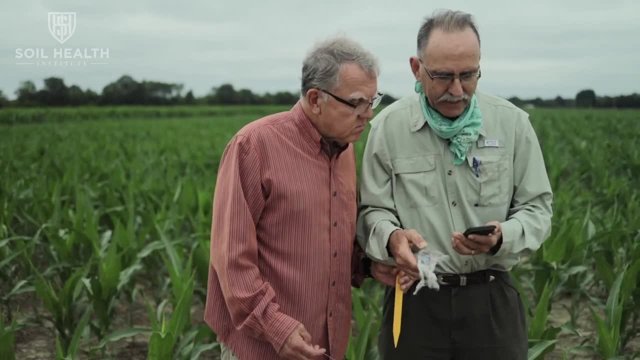 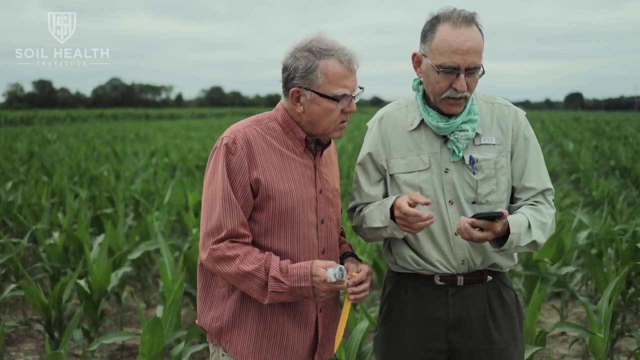 So let me just do that again And we'll get a shot of this. It's now 80.03.. And I'm going to save that for these guys. So we're going to deploy a few pendants. We'll put one really. 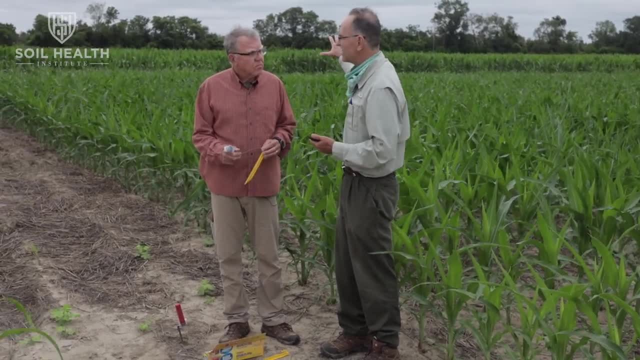 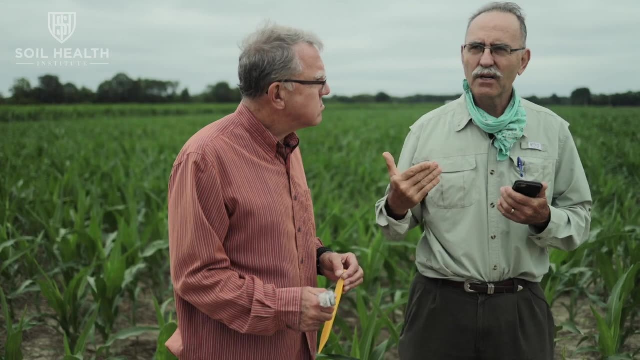 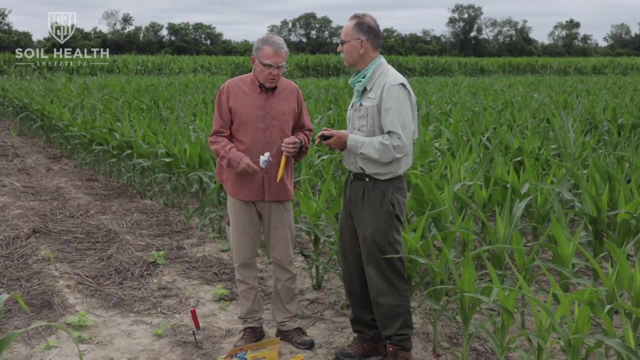 on bare ground. We'll put one under the canopy and then one a little bit away from the canopy, So we just wanted to look at that. We'll deploy them and then come back After we've had a few good sunny days. So do these measure like? take a measurement. 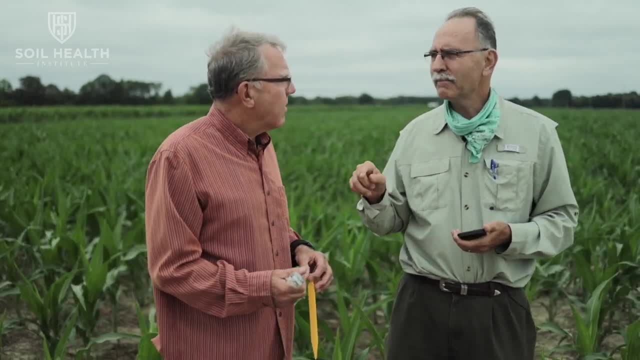 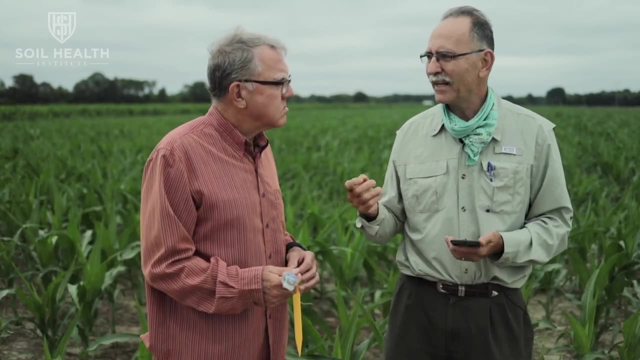 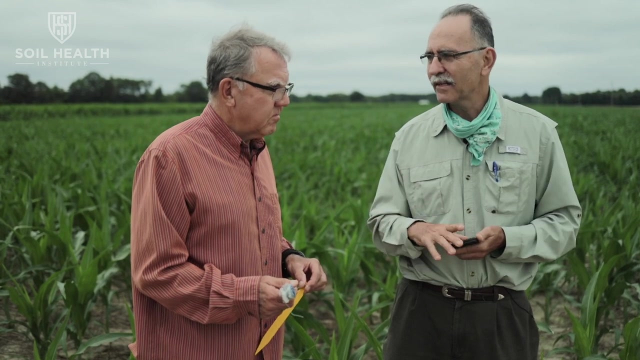 every 10 minutes or 20 minutes or something like that. Yeah, These are programmed to take a measurement every 10 minutes And then basically I can export that CSV file to my phone, Okay, And pick that up and then create Excel charts, And so it's really nice to be able to see. 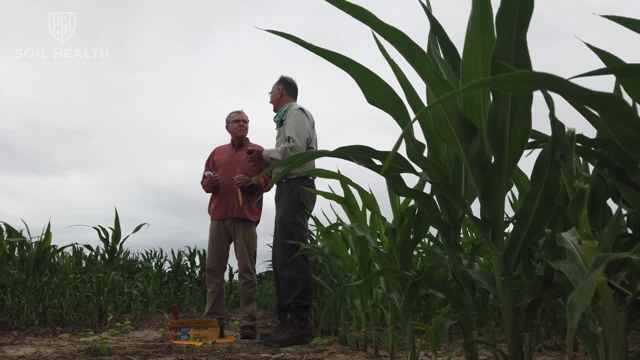 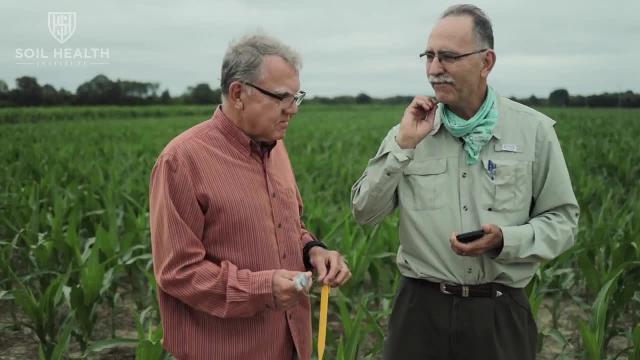 differences. Now, as a producer, why do I care what my temperature is? Well, think about walking on a beach, you know, at midday with bare feet. You're not going to be able to do that very easily. And in the same way, you know, once you get above. 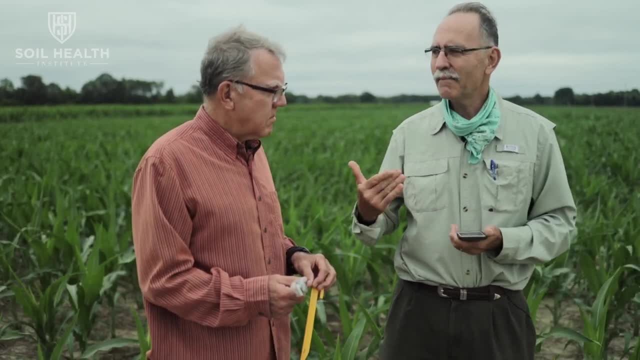 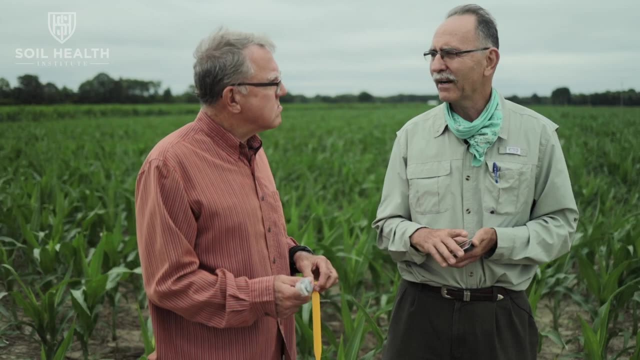 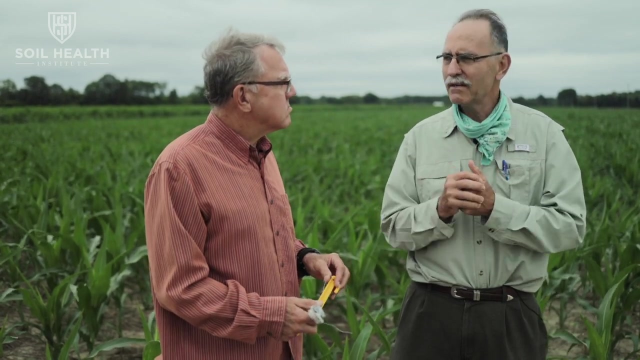 90 degrees and direct sunlight. you know your soil temperatures can go up to 120 degrees or more And that's going to kill off all but the toughest of microbes. You might have a few bacteria- Yeah, The thermophilic bacteria survive, but the majority of them are gone. So part of this 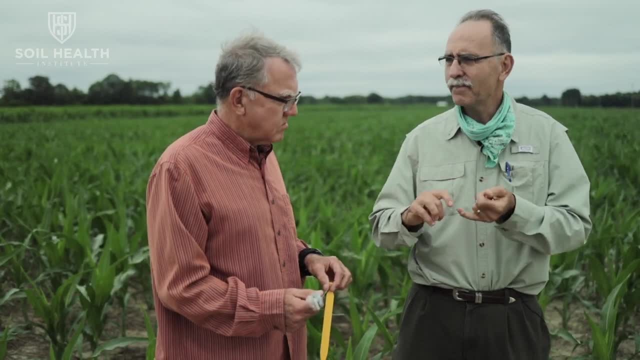 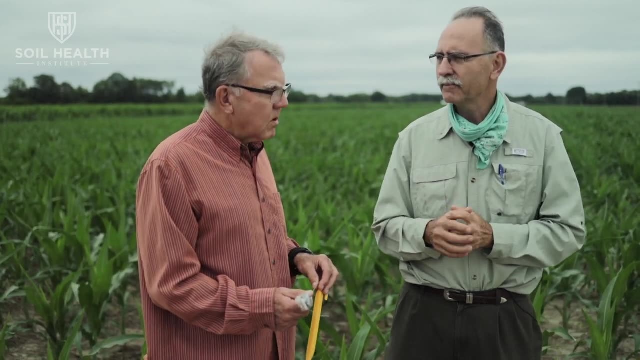 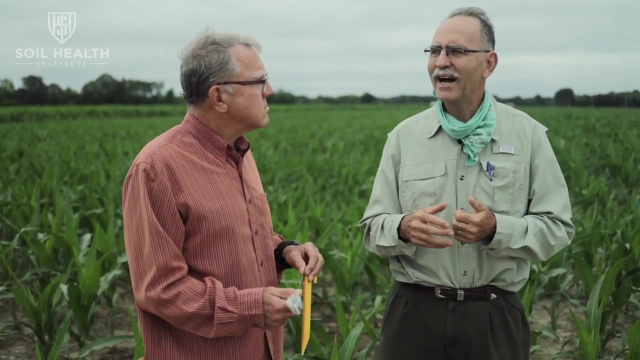 is part of the soil. health principles keep the soil covered with a canopy or with a layer of residue, So how does that affect evaporation? It's obviously going to put stress on the plant as well If you've got high soil temperatures. 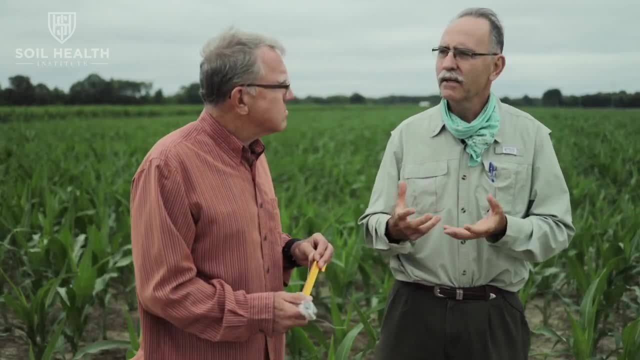 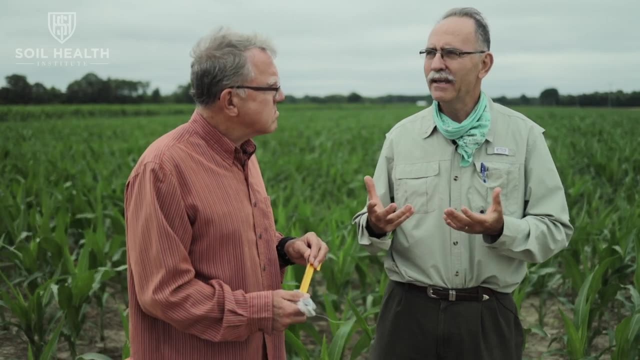 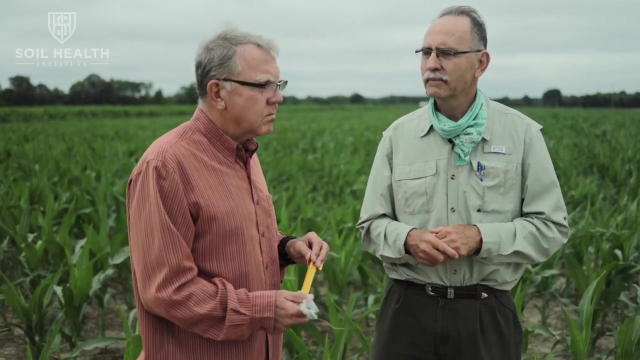 not only soil microbial, but then also it's going tovery high temperature, So it's going to increase evapotranspiration. more evapotranspiration is going to be a shorter time between rainfall events that your plants could dehydrate. This is a pretty simple test. Most farmers could do something like this. 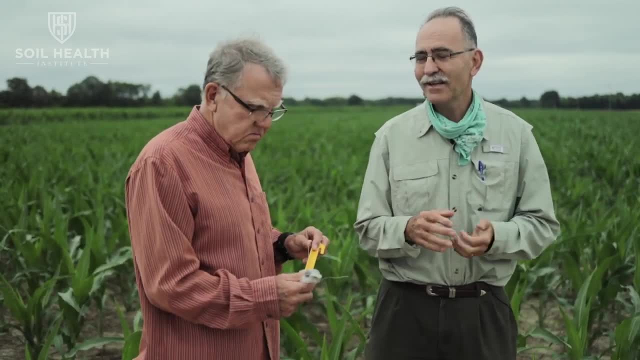 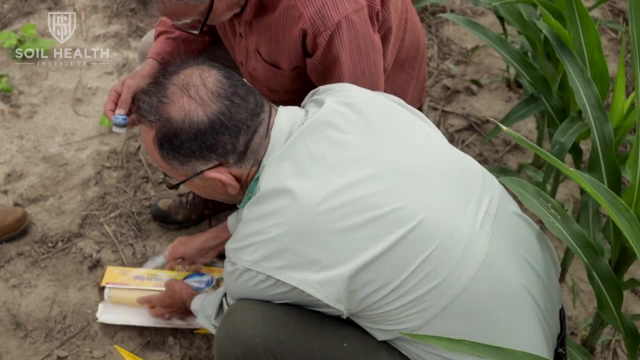 Yeah, I think that cost me like $57.. Okay, And so that's quite nice. Okay, One of the things. these are weatherproof, David, but I like to put a little bit of saran wrap around them. Oh yeah. 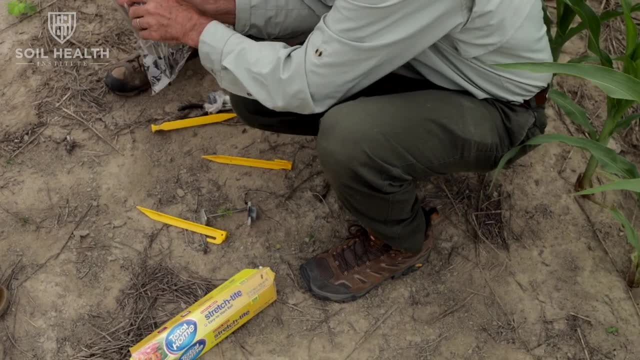 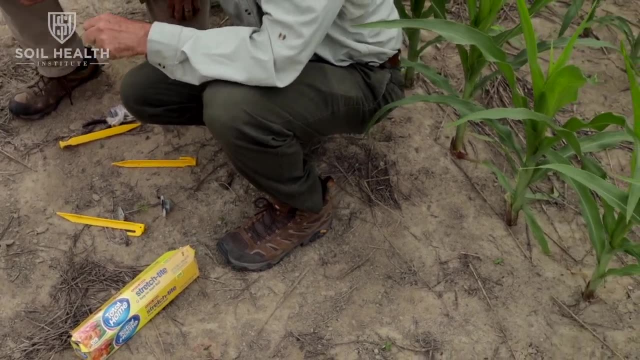 Perfect, Yeah, Nice. So this, there we go. we'll put the saran wrap around them and I'm going to put them in a couple of places. We've got some plots out here that we're going to put them in. 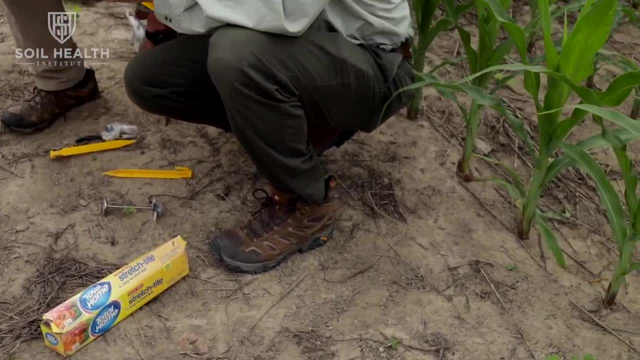 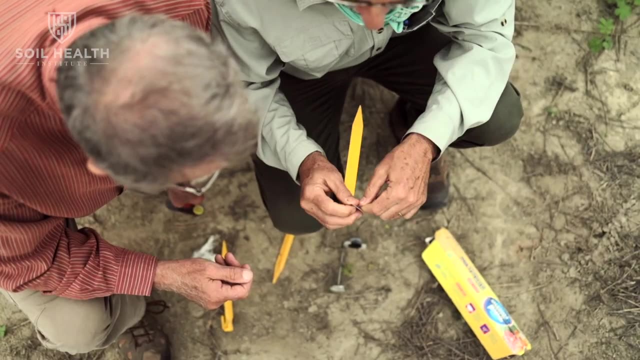 I'm also going to put something around them over here, a little tent peg, because, as you can imagine, these things can get lost in a minute. Yeah, I can. So there it is. Yeah, But to activate it again, let me just quickly. 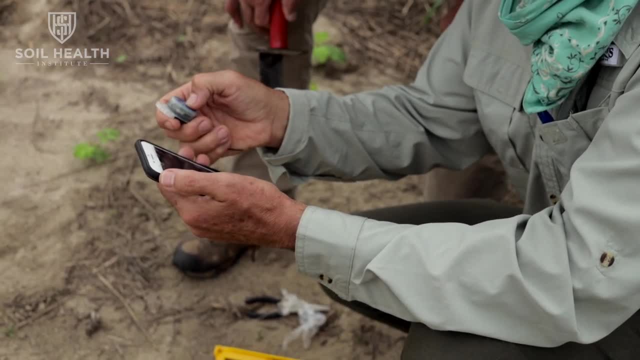 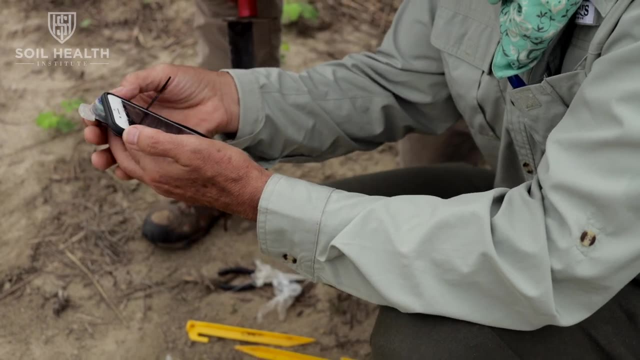 Now, are there other tools? Buzz, I mean, this gives you a difference. I'll probably give you. show you as it warms up during the day and cools off at night. Yeah, Are there other tools that we could use? 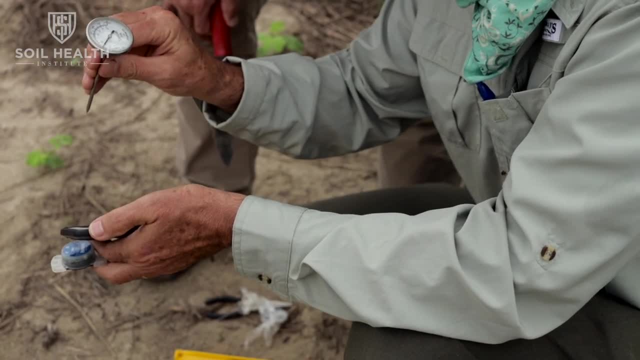 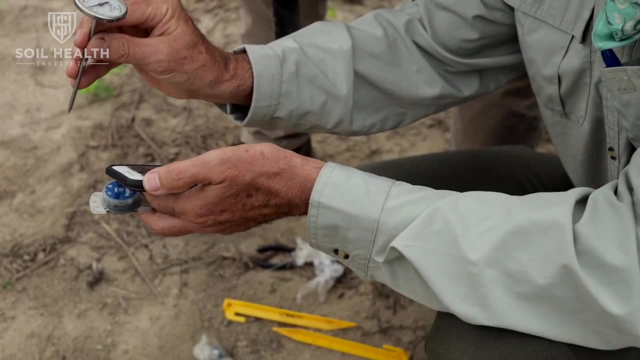 Well, you've got your simple soil thermometer. So this is an analog thermometer. So you know we use that a lot. I can't find my digital thermometer, which was really nice, But you just stick that two inches into the ground. 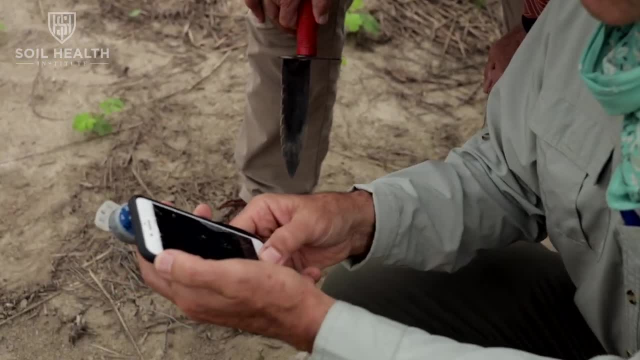 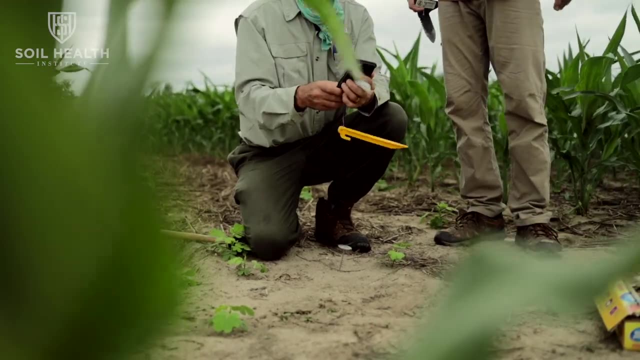 Okay, So the magic number is two inches as far as measuring the soil temperature, I think so. You know, that's not a bad. that's not a bad number. So all right, For the record. now I'm going to click on this one. 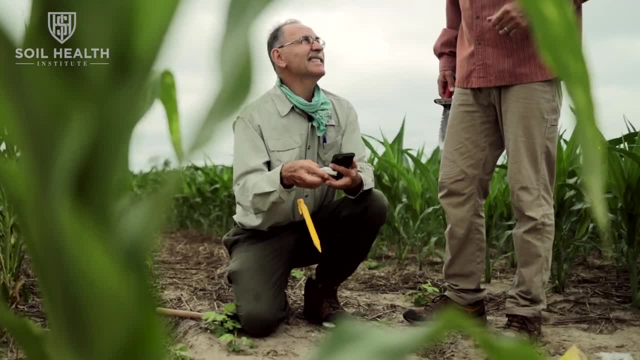 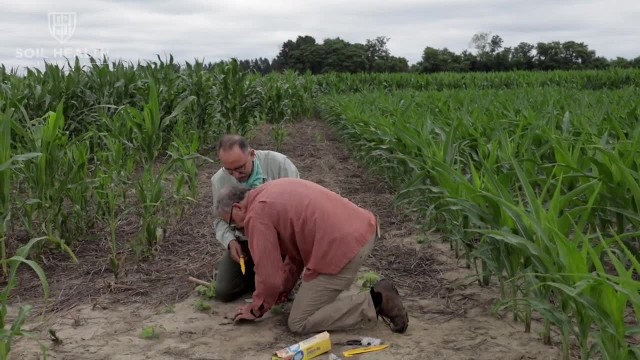 We're rolling, We're rolling. All right, David, this is NCO5.. Okay, And ambient temperature is 80.. Can you just dig a little hole for us please? There we go And we're going to stick it under there. 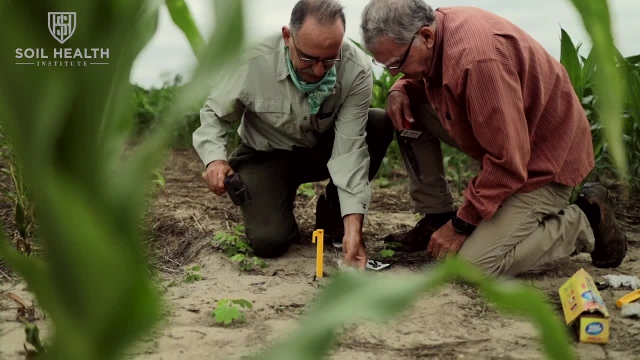 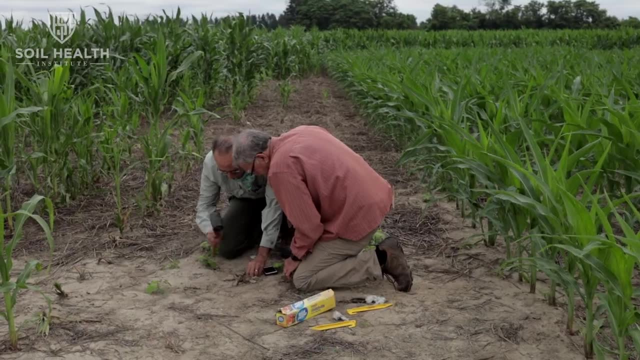 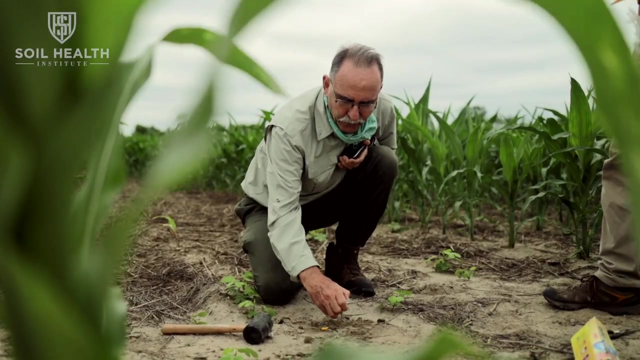 Okay, And I'm going to clobber this in so that the coyote is done. That's funny, Yeah, it is kind of funny. And then there we go. That should help us. Okay, And just for the record here, our temperature is about: oh, I don't know. 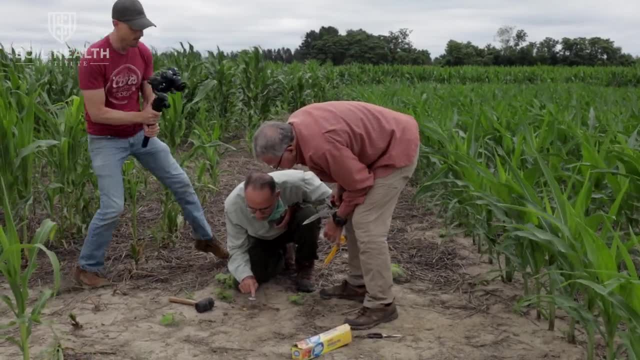 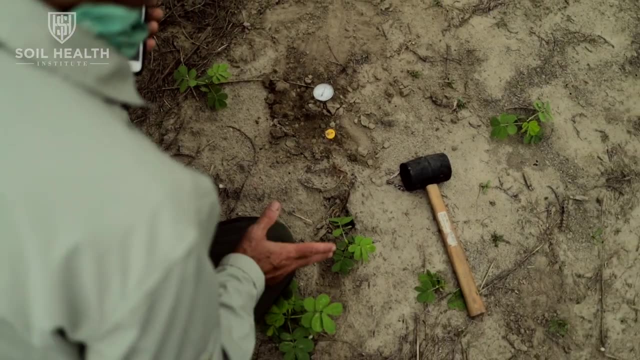 What is it? 40,, 50,, 60. About 65. So it's really cool right now. You know it's cloudy overhead, Okay, So we don't expect any temperature differences right now, Right now. 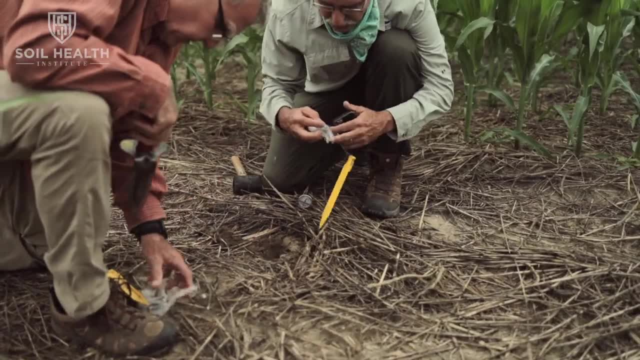 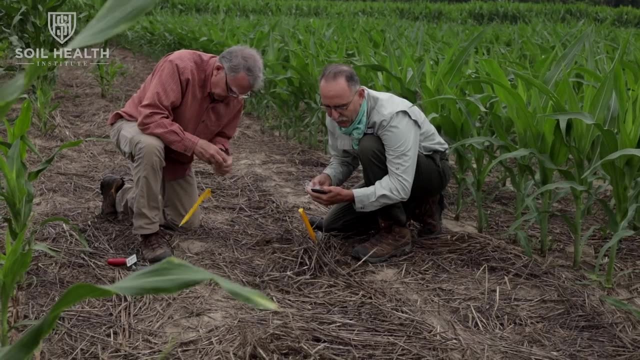 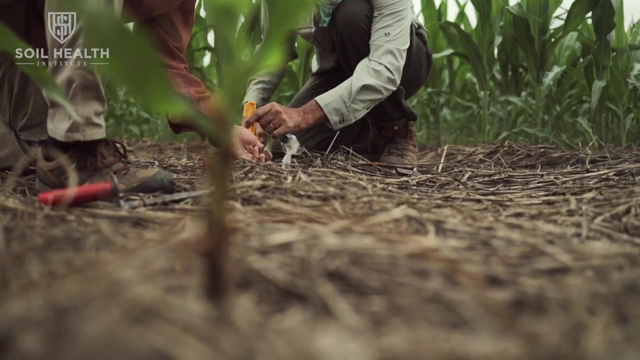 Yeah, Yeah. So let's have a look. This one will be NC4.. So I'm just going to activate: NC4 is on, So I'm going to drop it in here And clobber that in. Don't be so eager, David. 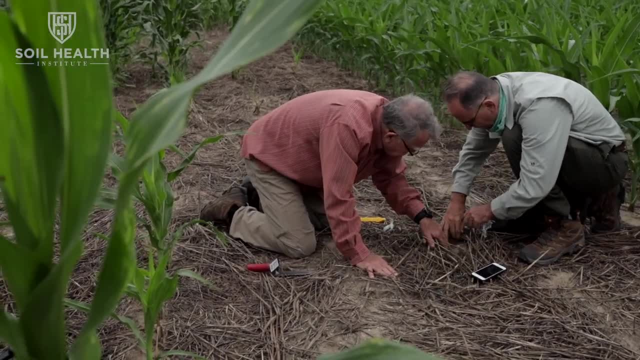 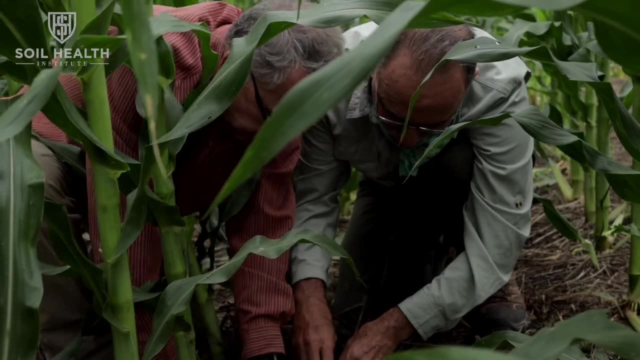 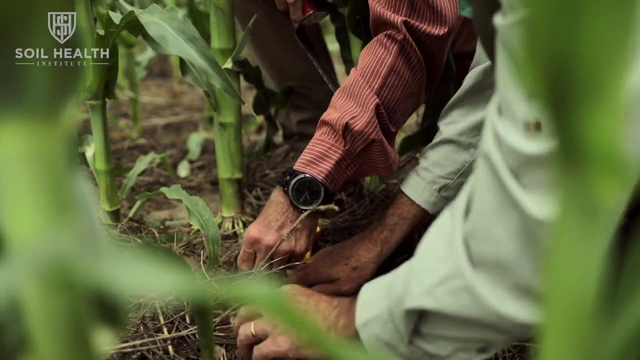 Okay, So pull that residue back. Let's bury that sucker in there. So now we've got a little bit of residue And of course we have a canopy. So we've got sort of three scenarios here And you know you're not going to get much of a difference. 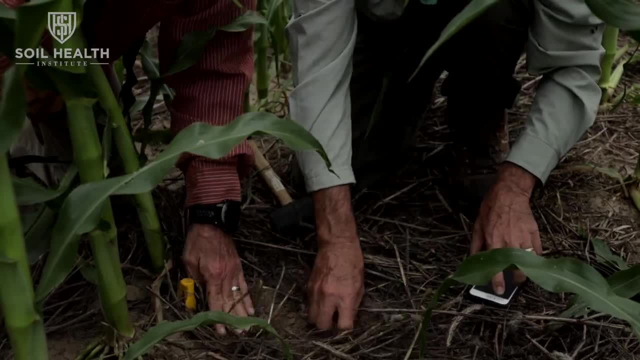 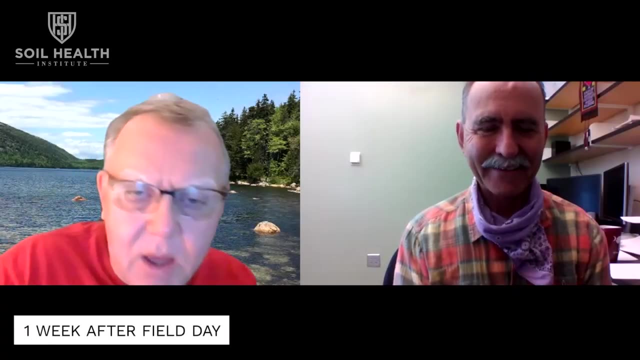 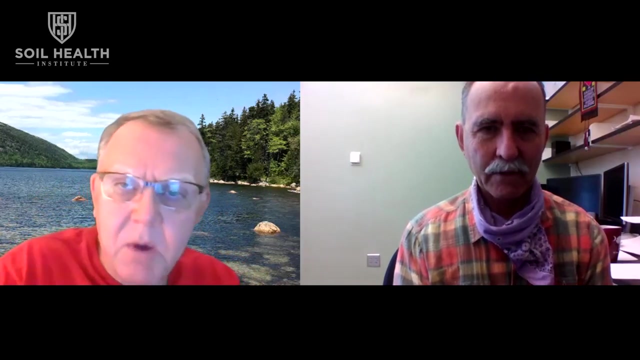 And hopefully the coyote is done coming. Pick it up, Pick it up. Hey Buzz, You've been out, You've pulled the data loggers for the soil temperatures And you've flooded up to the results. A period of time. 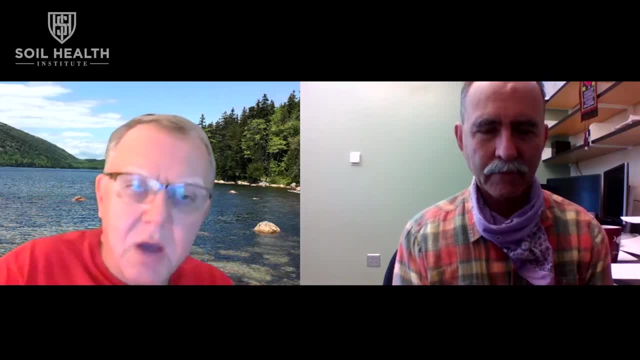 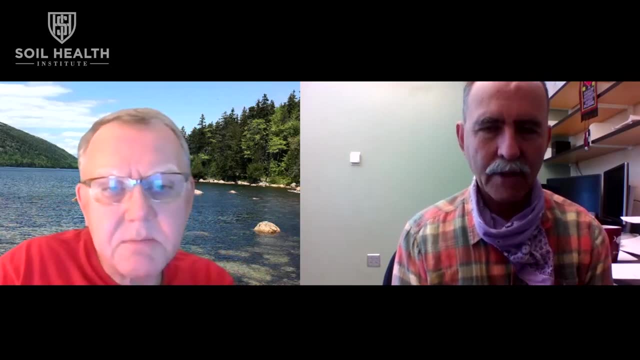 Why don't you kind of explain a little bit about what you found And then we'll talk a little bit more later about how that affects soil health function And maybe even how I get into a little bit of how it affects the property, If we just take a step back? 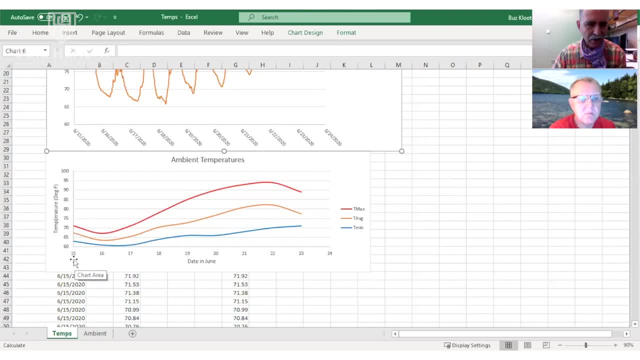 When you and I deployed those panels Pendant on the 15th of June, it was pretty cool and you can see our average temperatures were pretty low and high temperature even was below 60, which is unusual. And then over time, by the 22nd, our high temperatures were closer to 90 and 95 degrees. 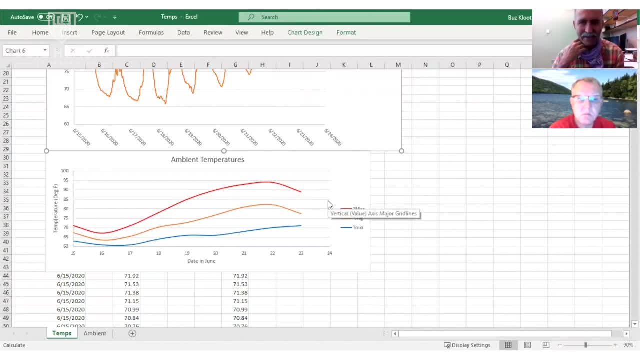 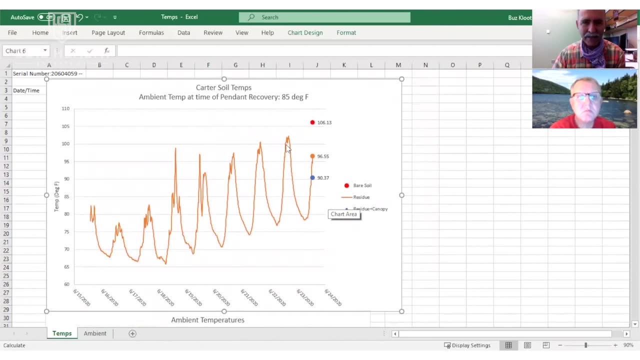 And then when I retrieved the pendant, the day that I retrieved the pendant, on the 24th, our actual ambient temperature was 85 degrees. So the good news is that the pendants, you know, we deployed the pendants. The bad news is that there was operator error and I only actually started the recording for the one pendant. 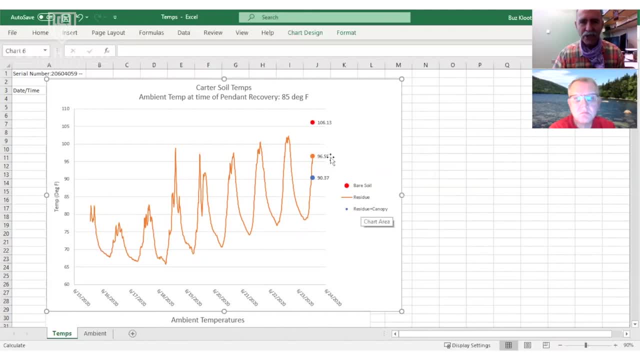 And that happened to be the one, The one in the middle, the one where we actually had some residue, the one under the canopy and the one in the bare dirt. we had nothing except those readings as we removed the pendants. So you can see just very quickly. under the residue you can see the fluctuations over time, sort of, with temperatures in the lows. you know, between 60 and 75, depending what your ambient temperature is. 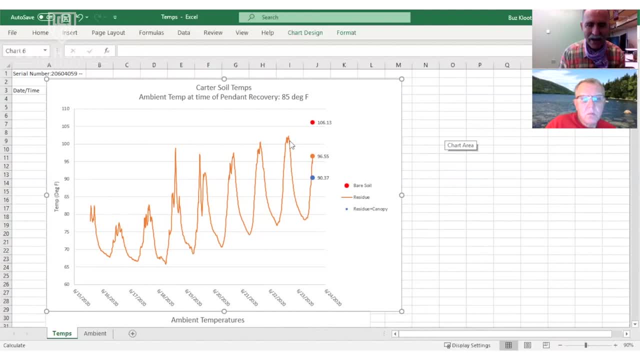 And then the highs getting up to about 100, so that was a residue that had no canopy. What was really gratifying about these readings? so this is: I suppose we're trying to be transparent. This is what happens when you have a field demonstration and you don't do your homework. 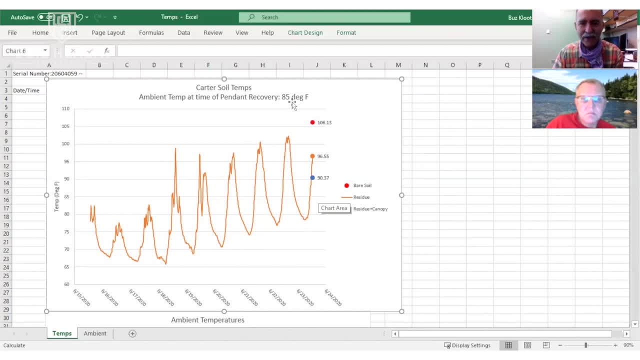 So that's on me, But I guess over here what you can see is our ambient temperature. The ambient temperature when I retrieved the pendants was about 85 degrees And at about an inch and a half to two inches below the ground we had 106 degrees in the soil. 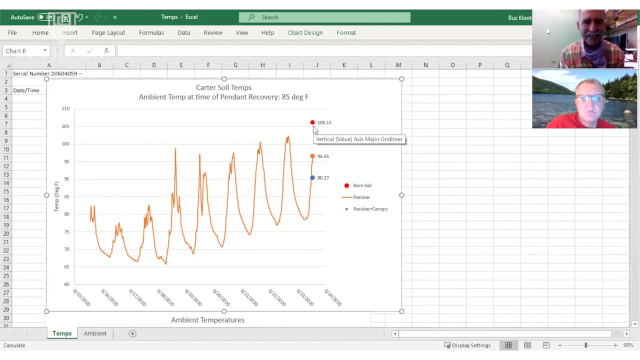 What was also interesting was that, you know, by sticking our regular analog soil probe in, it wasn't quite getting up to the sort of temperatures we were seeing here. We were seeing differences, But not that great a difference. So I think you know the soil pendants really pick up what's happening in the soil. 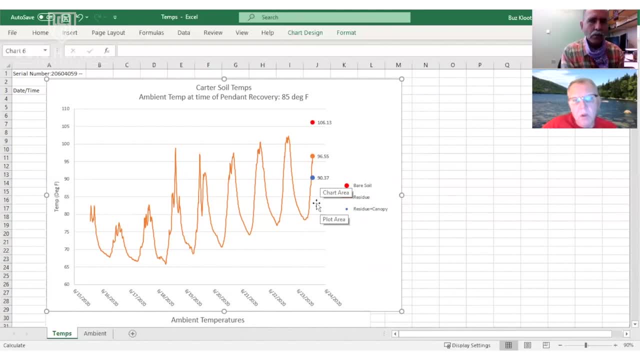 What time of the day were you gathering this? I'm just going to get a. how long of a period would we see these 100, 105 degree temperatures? Yeah, For like two hours, three hours. What are we seeing there? 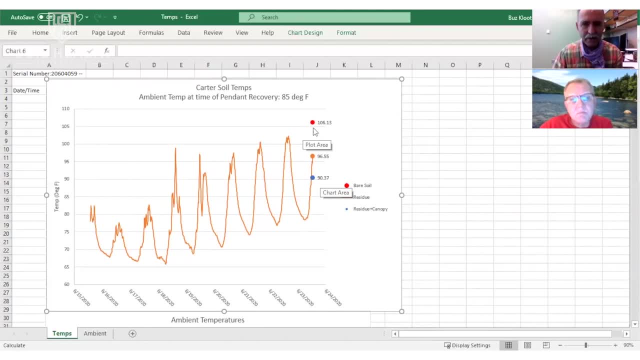 Right, I got my the probes over here at about. it must have been Two o'clock, So if you have a look here, let me just at this point: usually, as it's, it was still rising at by two o'clock. 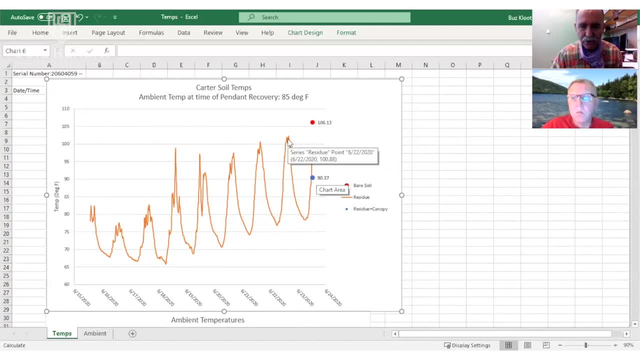 So what we see is usually by about 2.30 or three o'clock, And I'm guessing a little bit here, but that's probably when your soil temperatures begin to peak. So You would probably see temperatures if you have a hot day. 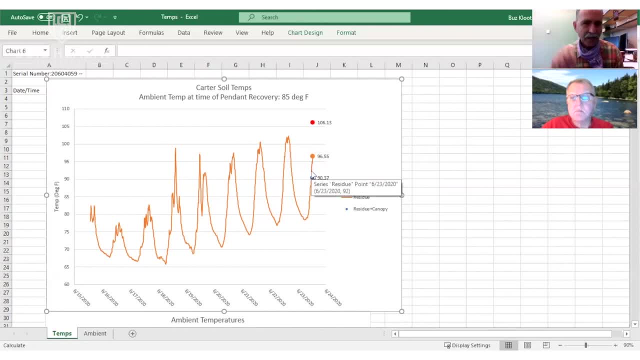 So keep in mind this: this was an 85 degree day. If you have a hot day, your soil temperatures are going to start peaking somewhere afternoon, And probably still go up, you know, and be in that high zone until 4 or 4.30 in the afternoon at least. 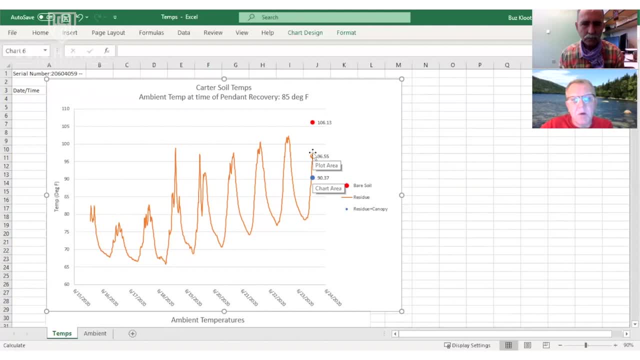 A little bit. Okay. So we know there's soil variability or temperature variability. We're seeing that's pretty significant. You got 26 degrees between where you had some residue in a canopy and where you had bare soil. What I mean? how does that play out? related to moisture, and maybe even a little talk a little bit about how it affects plant or crop production. 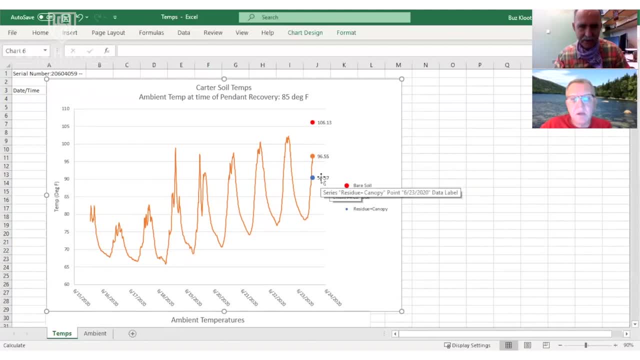 Yeah, So this is not 26.. This would be 16 degrees. Yeah, Yeah, Yeah. Well, I mean it. it just kind of goes to show How much residue, Residue and canopy protect the soil from sunlight. 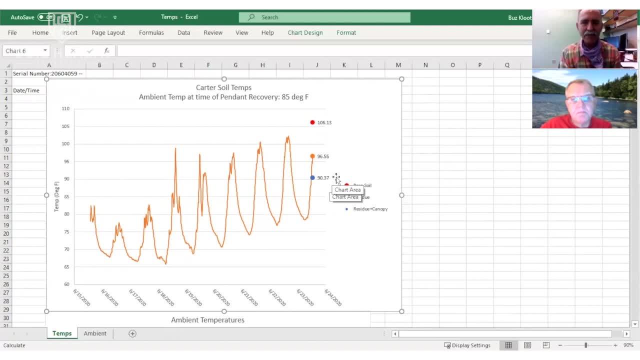 You know, we hear that theoretically, but here's some very good empirical data that that we can demonstrate. And so two of the things that we talk about is keep the soil covered either with residue or a canopy, You know. so, keeping the soil covered and- and of course that goes hand in hand with not disturbing the soil- 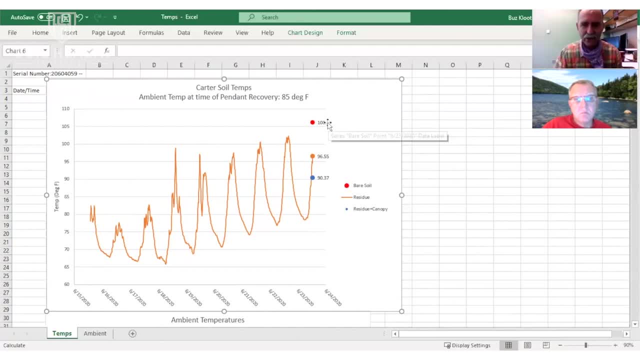 This is very evident over here. Okay, So this is a high, Highly disturbed soil where there's no canopy and no residue at all, And this is a a a soil with with little less disturbance and um um, with that canopy as well. 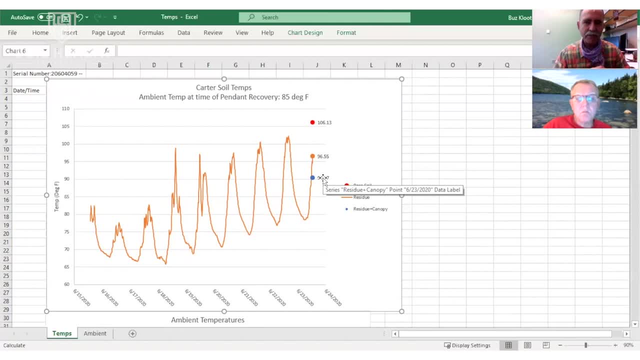 And you could see in the video. you can see quite a bit of residue. Well, I think we talked about when we were putting these out. we talked a little bit about how that affects those microbes that are most beneficial for for food and fiber. 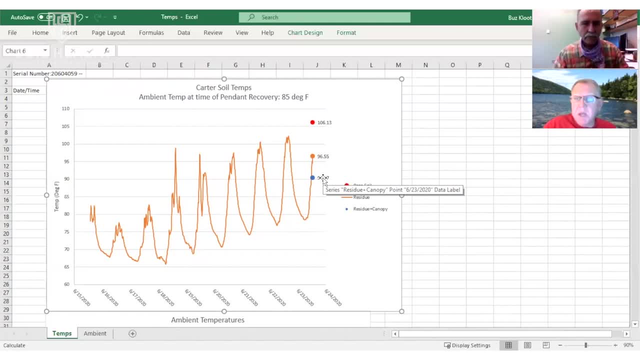 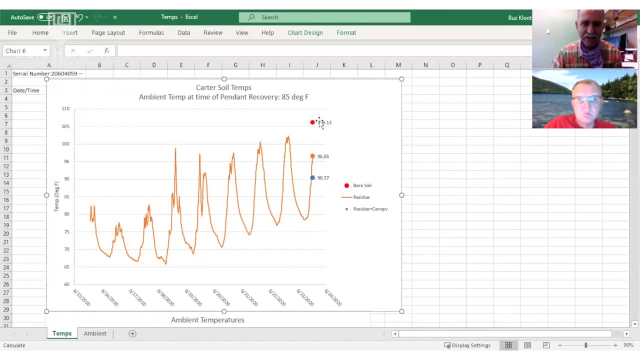 So, uh, I mean, as we we saw, we really don't have the soil that we were expecting. degree and above temperatures, all but your most thermophilic of microbes are going to either shut down or die, Or, you know, if they're lowered down, you know the soil temperatures will. 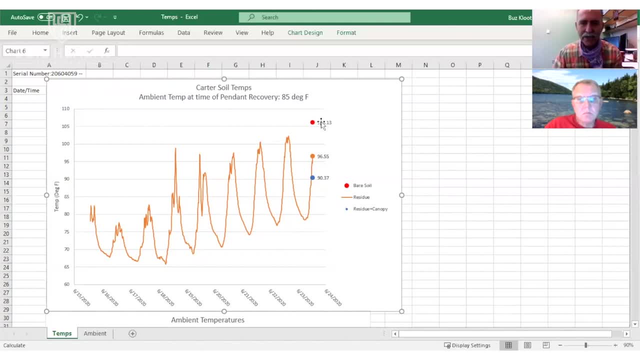 be lower, But in those top two inches you're going to shut down a lot of the microbiology over here or in all but the very, very thermotolerant microbes. So usually you know we talk about the optimum being in the 70 to 80 degree range And at this point 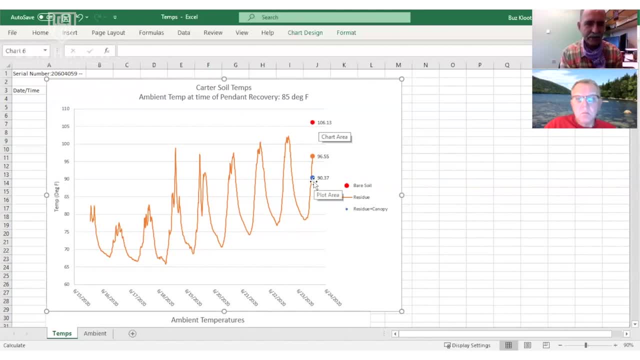 we're really out of that range. So it's just, you know your bacteria are probably going to stay around longer, And then your fungi. but protozoans and nematodes- those guys that sort of- are responsible for eating bacteria and fungi. and then 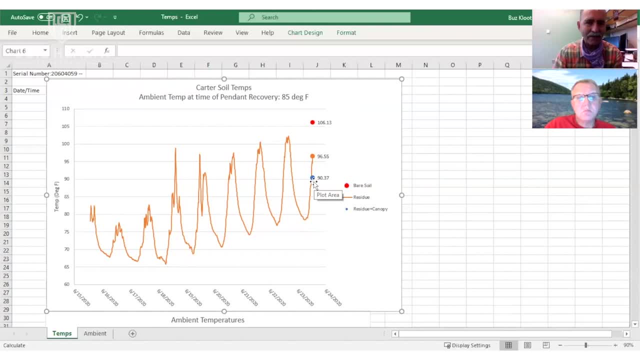 redistributing nutrients. you're not going to see many of those at these temperatures. Okay, Well, listen, Buzz. I think this is really interesting. These are something a farmer can do with a simple thing: Go out and get a. maybe not use a pendant, but they can actually use a soil. 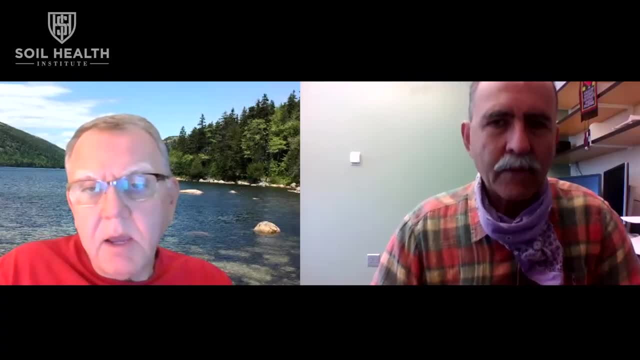 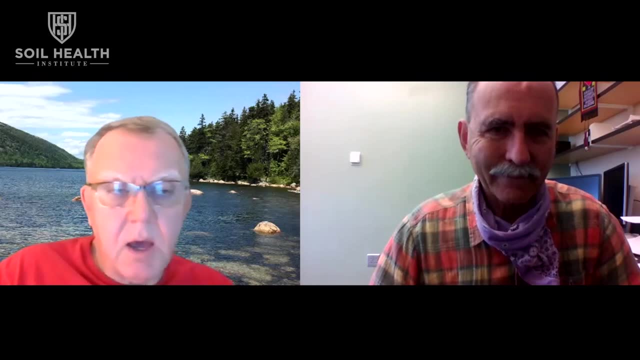 thermometer. They're easy to get and kind of go out and play around on their own, And I guess I'm trying to lead into those who are. we're going to have a video here talking a little bit about soil biology and looking at those critters that you just mentioned. 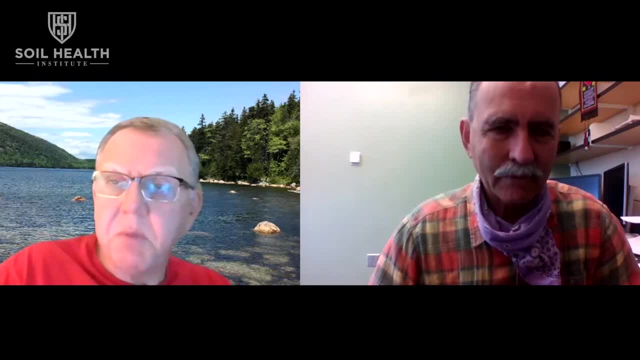 Under a microscope. So I just encourage those folks to participate, join in and watch the next video in our virtual field day series. So thanks a lot, Buzz, and we'll have more to come. Thanks, David, Good to talk to you and we'll catch up later.